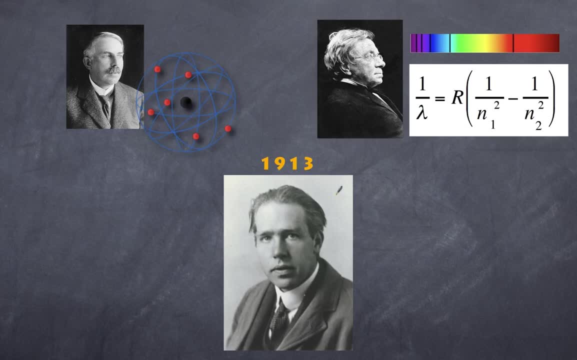 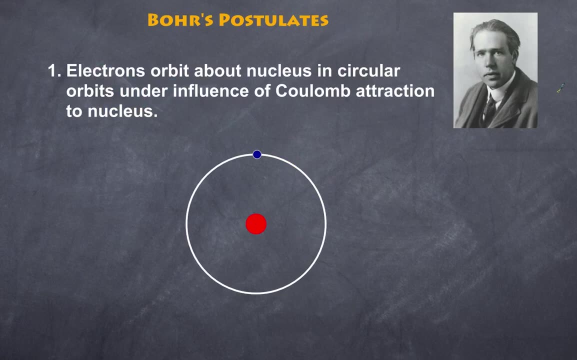 explain it, but, as we'll come to see, Niels Bohr is able to explain that. So let's get started. Well, Bohr basically came up with some key postulates, and we're going to examine them one by one. The first thing that Bohr's postulated is that the electrons 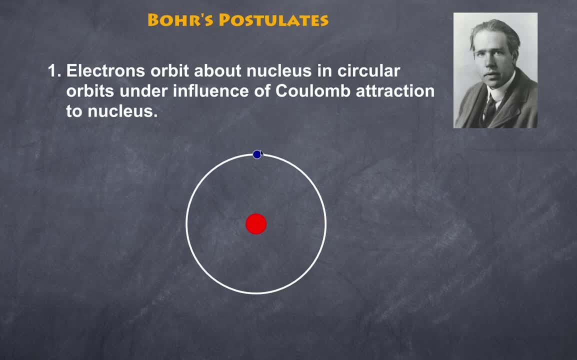 orbit around the nucleus in a circular orbit under the influence of Coulomb's attraction to the nucleus. So in that regard we are no different to what Rutherford already stated. He was consistent with Rutherford's view that the nucleus was in the center and most of the mass was there and that the 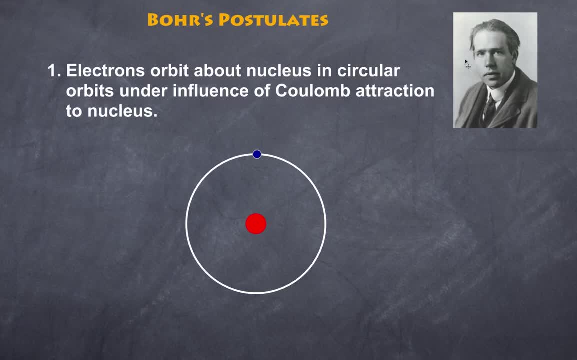 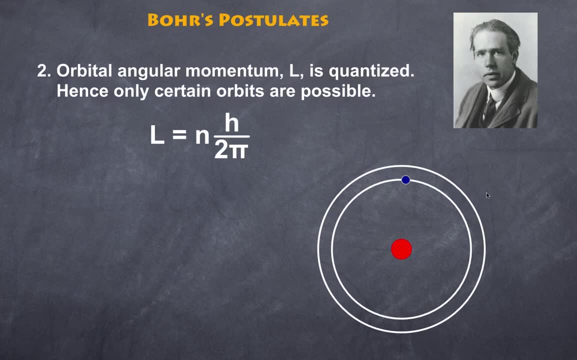 electrons were in orbit around that nucleus. The second postulate is really critical And if you look at your history of physics you know that in 1900 and 1905, we have the introduction of quantum thinking, initially with Max Planck's. 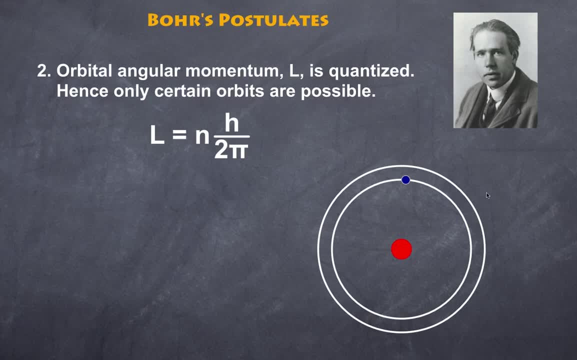 work on blackbody radiation and of course Einstein's work on the photoelectric effect, And Bohr took that on board. So he came up with the postulate is that electron here has angular momentum, which is L, And he's saying it is quantized. that is the amount of angular momentum. 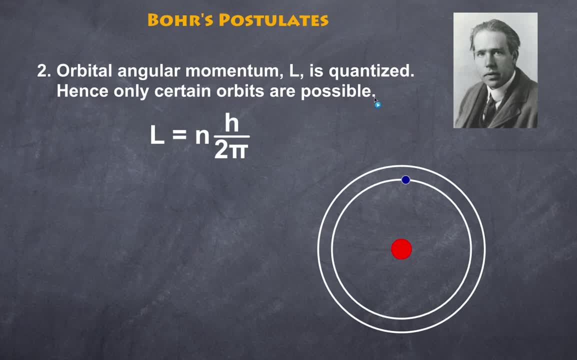 it has is a set value, And so therefore only discrete orbits are allowed. And this formula was the formula on angular momentum, So n was simply a number: 1,, 2,, 3,, 4, 5 integers for each. 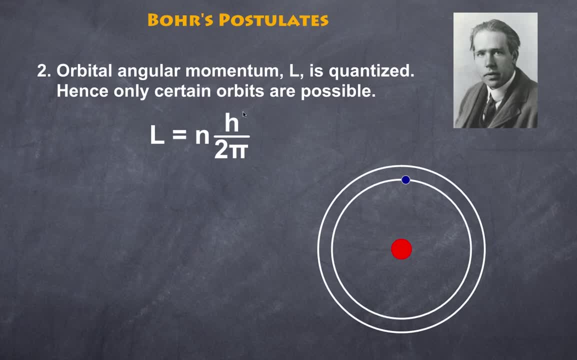 of the levels here that we have. h is Planck's constant, which we are hopefully familiar with, and 2 pi, of course, is just a constant. So basically, what he's saying is is that this electron can exist in this orbit, this electron can exist in this orbit and this electron can. 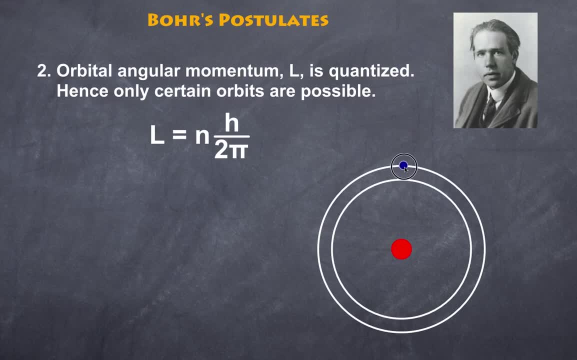 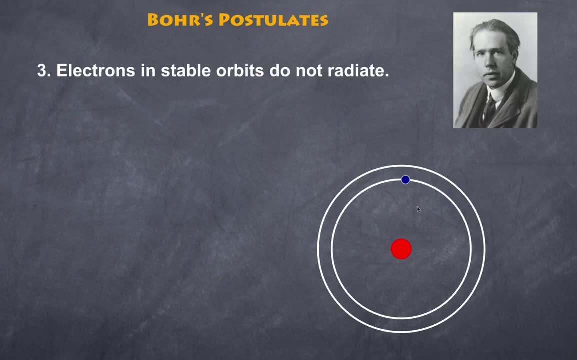 exist in this orbit. but it is impossible for the electron to exist anywhere in between. So it was a quantized value or discrete. Tied to that is that if those electrons are in an orbit, in this case in that particular orbit, as long as it stays in that orbit it actually does not radiate any. 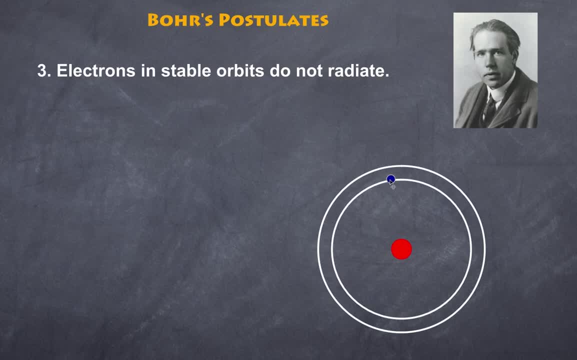 energy. In other words, there is no gain of energy, there's no loss of energy. If the electrons was in this orbit, it also would be stationary. So if the electrons were in this orbit, it also would be stable. And so that's the third postulate, That is, the electrons, as long as they're in one orbit. 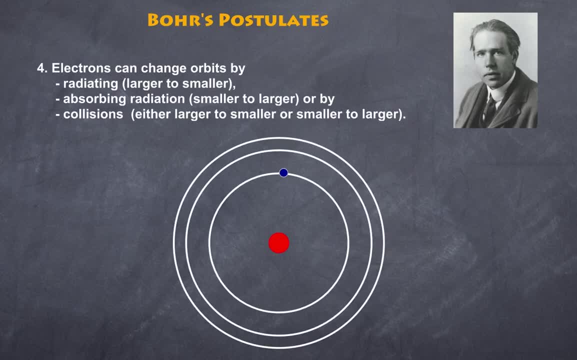 will not radiate any energy. Now, this is the critical one. Basically, Bohr said: okay, how can an electron go to another orbit? Well, the first thing that they could do is they could be radiating, So they go from a larger to a smaller. So if, for example, my electron is sitting in this orbit, 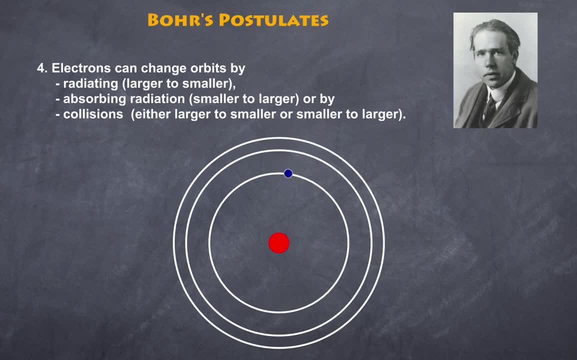 and it moves to this orbit, then what will happen is it will radiate energy as a result, Because the energy here will be higher and the energy here will be lower. So E2 minus E1 will mean a certain amount of energy, and that energy 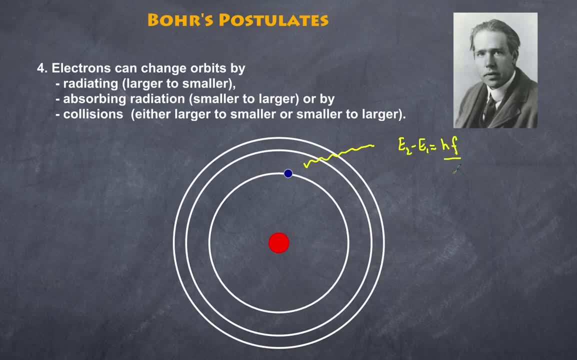 will all be quantized. E equals HF. The other thing that often can happen is that the electrons can absorb energy, But again the amount of energy that they absorb is an all or nothing thing. So let's say E1 is a particular amount that allows it to go to this particular orbit. But if the energy is slightly 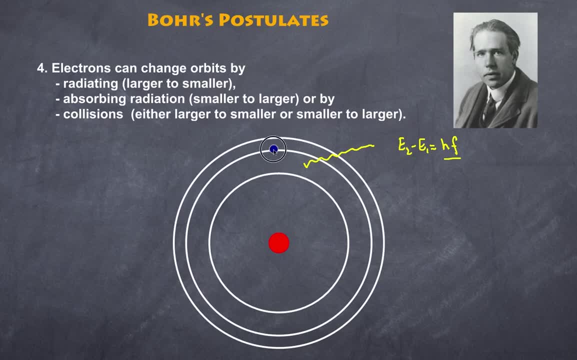 greater but not great enough to get to this orbit, then the electron will stay in this orbit. So either it moves to this orbit, or it moves to this orbit, or it just moves to that orbit. It can't sit anywhere in between. And lastly, these electrons can change orbit by collisions, So in other words, going up or down. 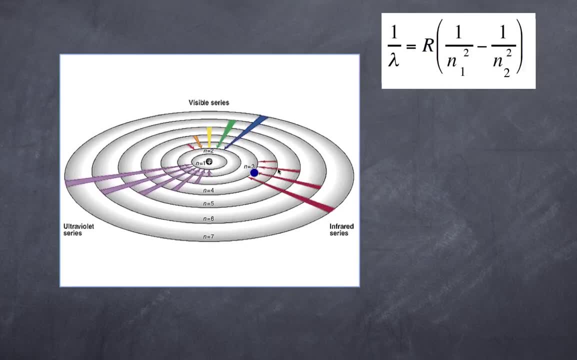 through two collisions with other atoms. And here is where Niels Bohr had a great insight. Remembering Rydberg's formula, which is sitting up here, he was able to explain why the emission lines, or absorption lines of hydrogen are the way they are. 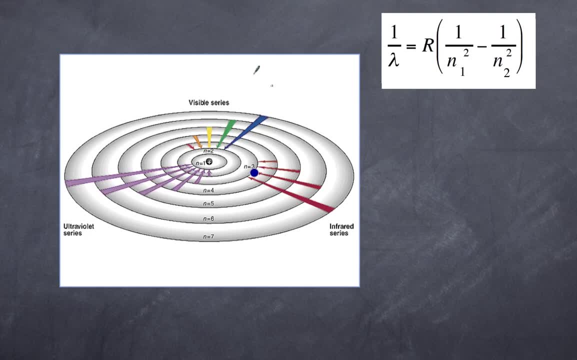 Now, initially, of course, we're going to be looking at the Barmer series, And the Barmer series are the hydrogen lines that can be calculated using this formula, that therefore give us these lines in the visible part of the spectrum And, if you remember, the 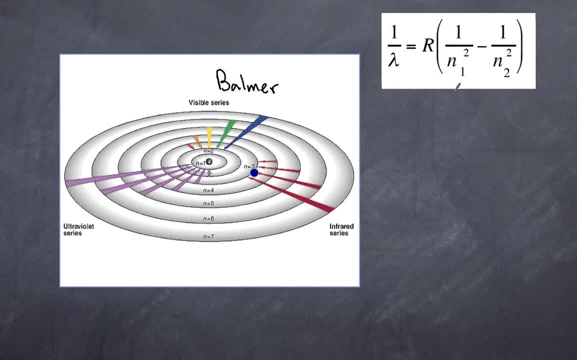 value for the N1 ends up being two in this case. So Niels Bohr said: Well, I can explain. why this is the case is because if atoms of hydrogen are absorbing energy and those electrons are jumping to high energy levels, then those electrons can jump down back. 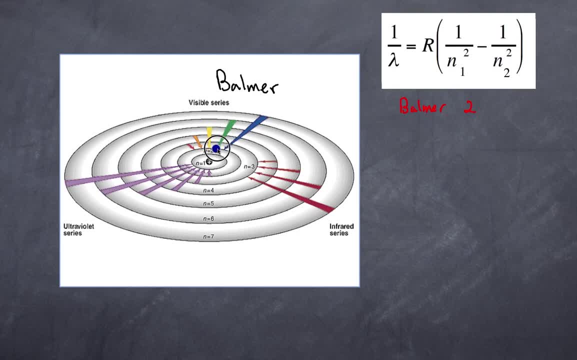 down to level 2 and release very discrete amounts of energy. That is, if it jumps from, let's say, N3 to N2, then of course what you would get here is a wavelength that would correspond to the red part of the spectrum. If you would jump down from N4 to down N2, this would become 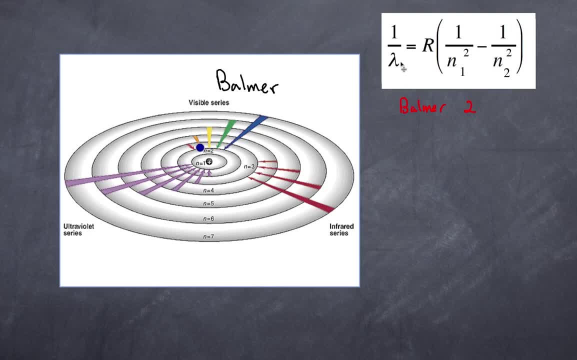 4 over here. This wavelength, therefore, would become smaller and, as a result, you would get a higher frequency and it would correspond to orange and so forth. That would explain why you get these lines. Now you not only have these Balmer series, there are also hydrogen. 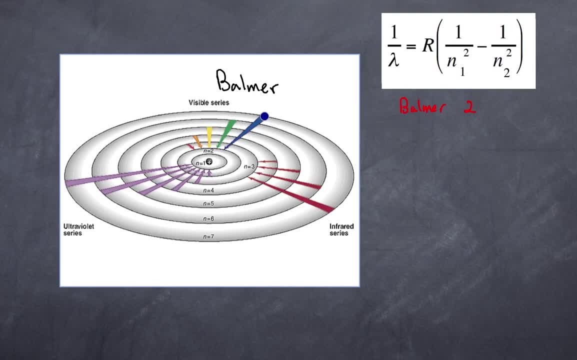 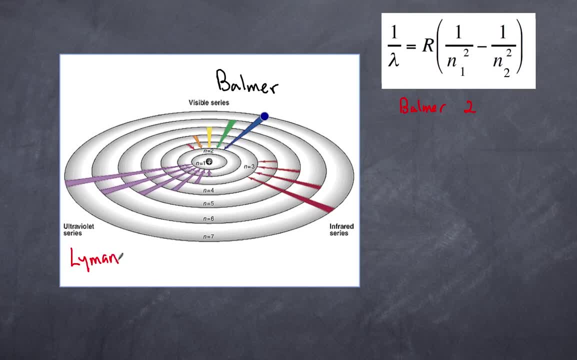 thing. The ultraviolet series are referred to as the Lyman series, whereas the infrared series are called the Passion series, And what that means is that instead of the value 2 being the first value here for the Lyman series, you get the N value being 1.. For the 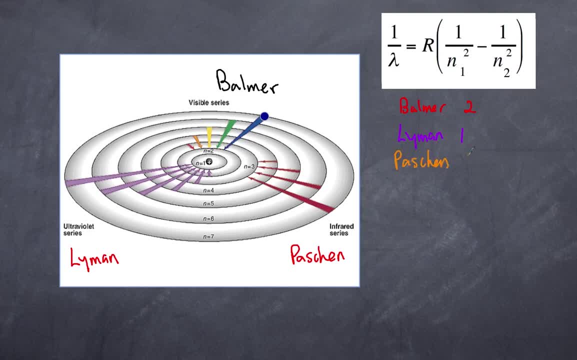 Passion series, you get them jumping down to 3.. And if you did the calculations using Rydberg's formula, you would see that these values here would correspond to lines in the visible spectrum. These wavelengths here would correspond to lines in the ultraviolet section and the 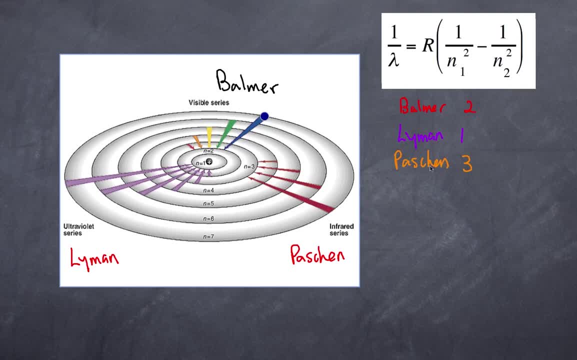 passion would correspond to the infrared section. So now we slightly modify the formula. So here's our formula again, but what you notice now, instead of 1 and 2, what we have is NF, which stands for final, and NI being the initial, And so if I have my electron moving, let's say, from this shell over, 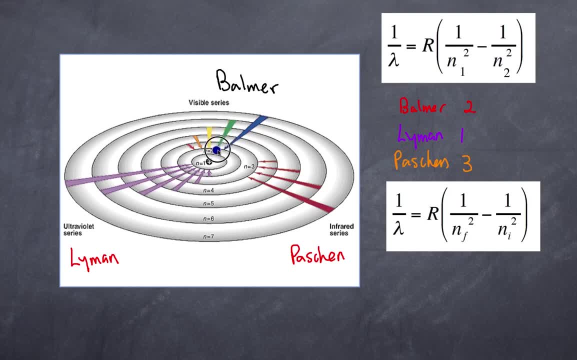 here, that is N6,, it moves down to N2, so my final is 2,, my initial is 6, and the green would represent the wavelength that I would get in that calculation And so using an understanding of spectral lines, 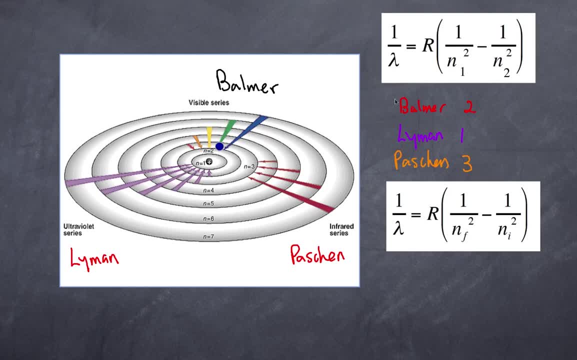 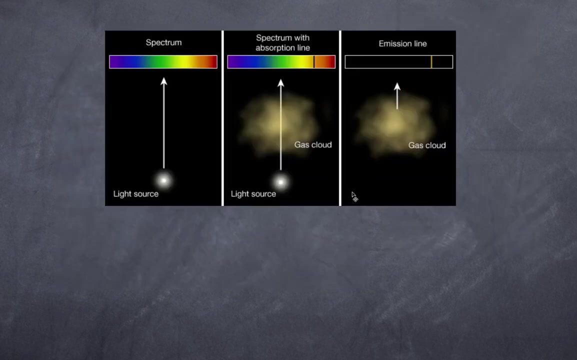 Bohr was able to verify his postulates in terms of the model of the atom. So now we have a model of the atom that is far more robust than Rutherford's initial atom, and it introduces the whole idea of quantum mechanics, because we have discrete energy values here. As I said to you, it could explain our 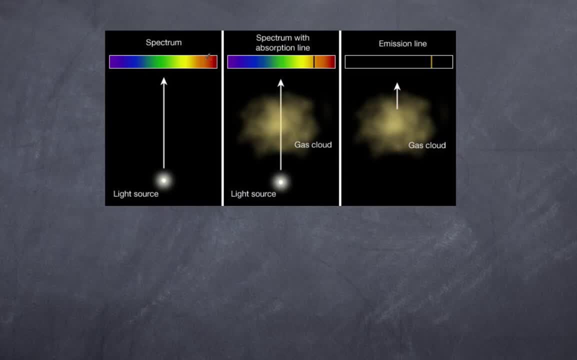 spectral lines. Here's my light source. I'm not getting any lines, I'm getting all the colours of light. But, of course, what is happening? here? within my gas? I have these atoms that are absorbing the light, absorbing the radiation, and the hydrogen atoms are of 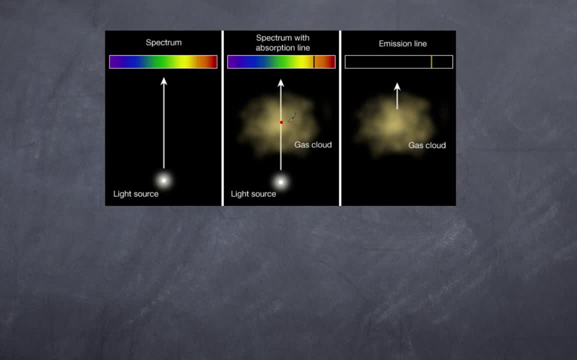 course, are reemitting certain wavelength And it's in a random direction, so they may go in a different direction, which means if you were to analyse this from over here, you would find these ones missing, because these are a very specific value HF. Similarly speaking, if 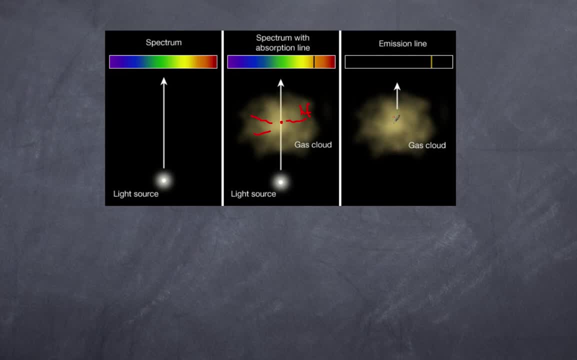 energy is within the gas cloud over here. the only energy you would get out is what is being actually emitted by my hydrogen gas, and again, that would correspond to the wavelengths due to the electrons jumping down various energy levels. so here we have supporting evidence for Niels Bohr's work. 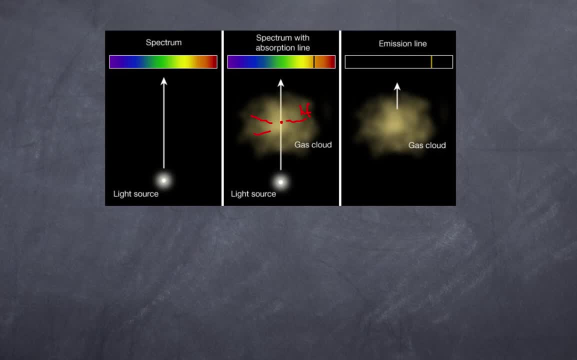 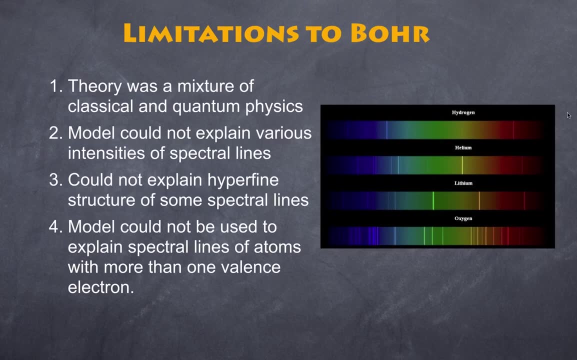 however, Bohr's model does have some problems, and we're going to look at them. the first thing is that the theory that he devised was actually a mixture of classical and quantum physics and, if you understand quantum physics, quantum physics supersedes classical physics, in other words, 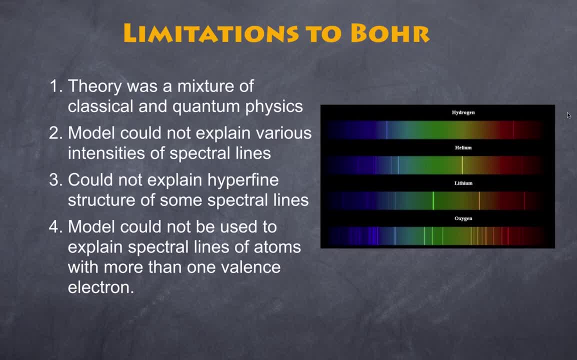 understanding of quantum physics explains everything we already know in terms of the classical sense, and so, by incorporating some classical understanding, it wasn't necessarily a valid way of looking at the model of the atom. secondly, the model could not explain various intensities of spectral lines. you'll notice some. some lines are of: